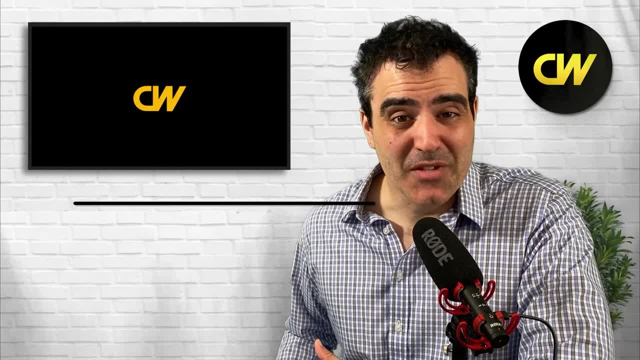 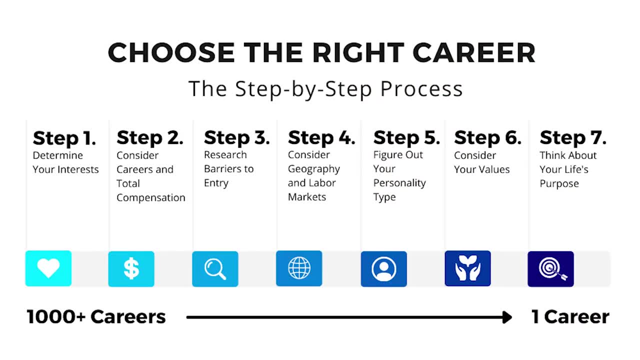 world a better place. Working in an occupation where you have a lot of job satisfaction is important. That's why we created a program called Choose the Right Career. It is a seven-step program to choosing the right occupation for you. We look at how much money you want to make. 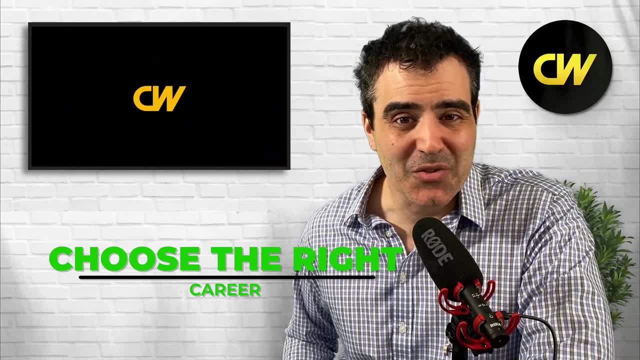 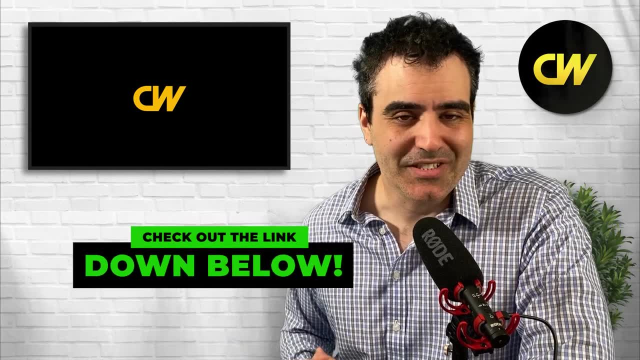 where in the country you want to live, your interests, your personality, your values and different labor markets, And we use all these different things to help you choose the right career for you. Check out the link below for more details. Like many of the other engineering 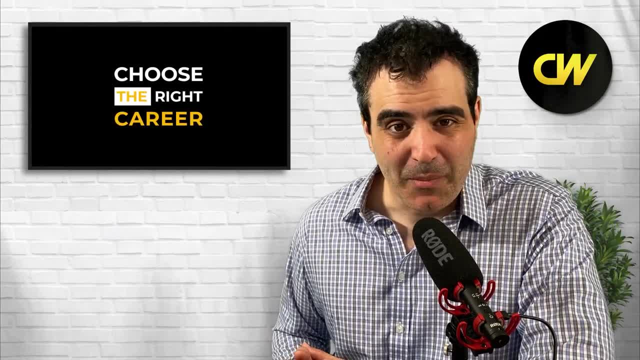 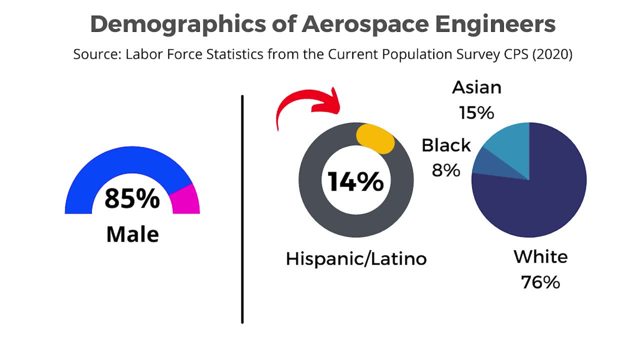 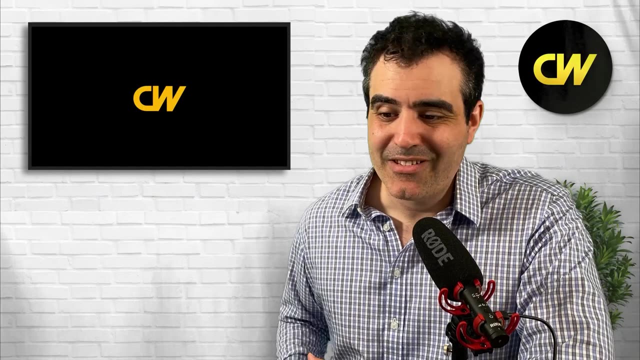 fields. aerospace engineering is a pretty male-dominated occupation. In fact, 85% of surveyed aerospace engineers describe themselves as male, about 14% Hispanic or Latino, 76% white, 8% black and about 15% Asian. 85% is pretty high, but there's actually quite a few other. 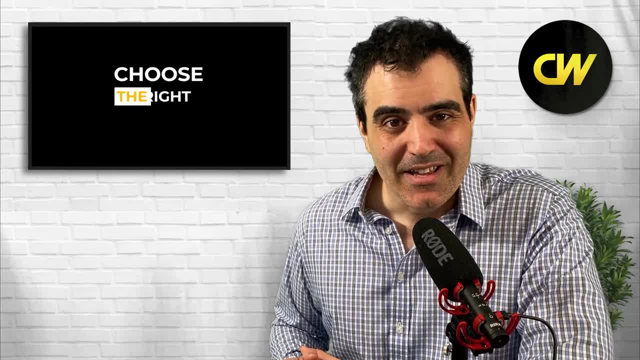 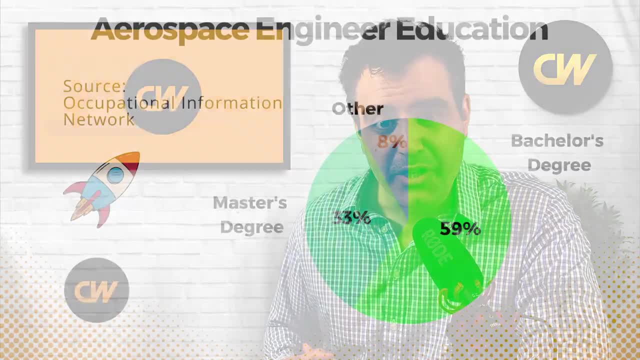 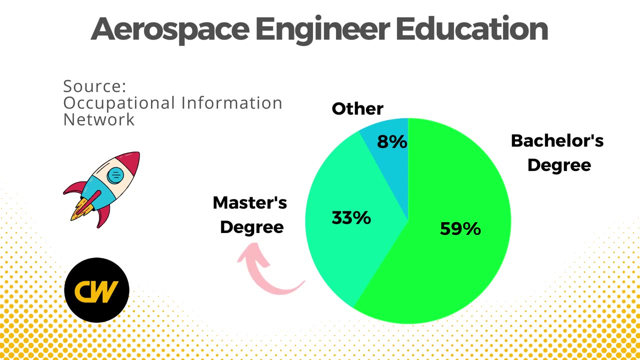 engineering fields that are way more male-dominated than aerospace engineering. First, we're going to talk about educational requirements and barriers to entry to becoming an aerospace engineer. According to the Occupational Information Network, 59% of aerospace engineers that are employed have a bachelor's degree. 33% have a master's degree. 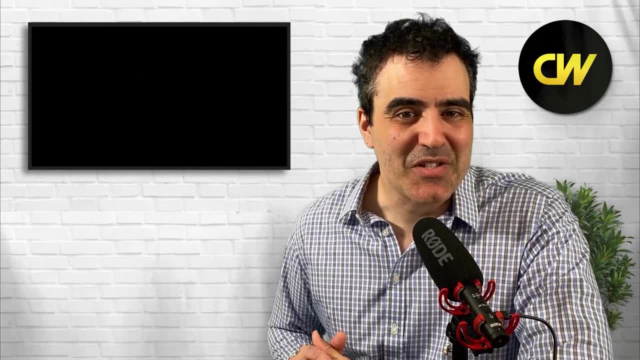 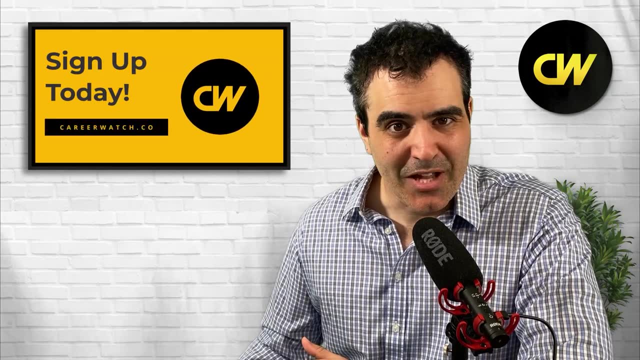 and 8% other. So one out of every three aerospace engineers has a master's degree. And you don't see this in chemical, you don't see this in civil, industrial, any of the big three engineering fields. Aerospace engineers tend to have a lot more education than many of 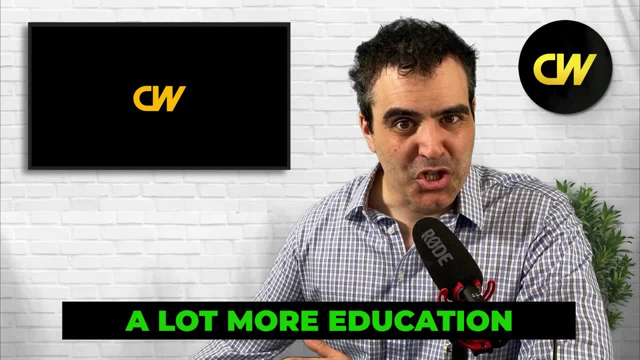 the other engineers, And so we're going to talk about educational requirements and barriers to engineering fields. In fact, one of the big advantages to going into engineering is often you just need to get a bachelor's degree to get most of the job opportunities. So this is kind of a con for becoming an aerospace engineer. Another potential con is the fact that a lot of aerospace engineering job opportunities require US citizenship. And it's not just the US citizenship, it's the fact that a lot of these job opportunities require a clearance And a lot. 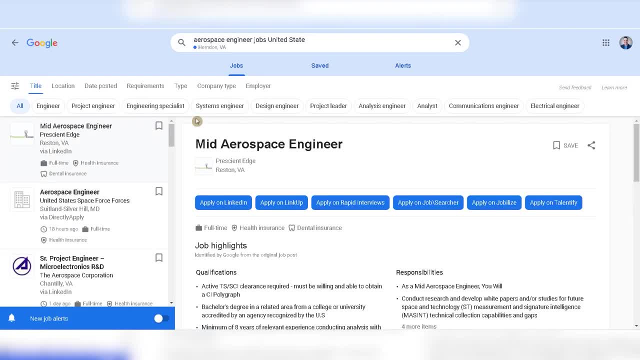 of people actually can't get government clearances. Even US citizens- a lot of US citizens- can't get government clearances. So what you see is when you look at a lot of these job postings- I'm using the Google search engine. they have a great job portal, But whenever you see something, 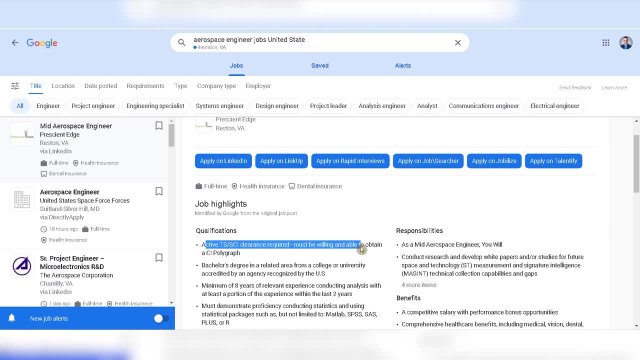 like active TSSCI clearance required must be able and willing to obtain a CI polygraph. A small part of the population can actually do this. I mean, if you have something like 33% of Americans have some kind of criminal record, whether it's a misdemeanor or felony debt. if you have foreign 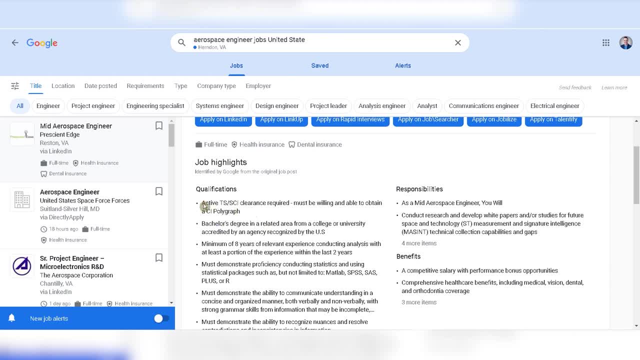 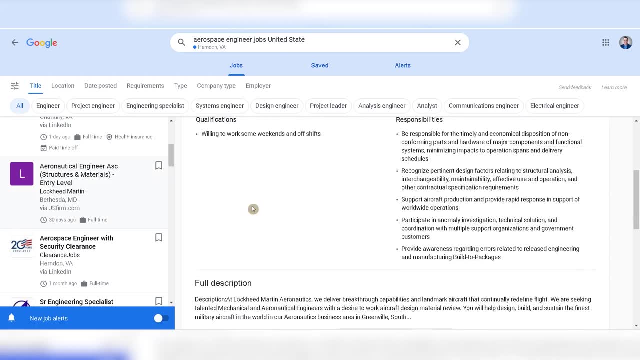 relatives. all this can prevent you from getting a TSSCI clearance, And this is a high level of clearance. But even lower level clearances can be challenging to get, And if you just look at some of these job postings, Lockheed Martin is a defense contractor. this most likely requires 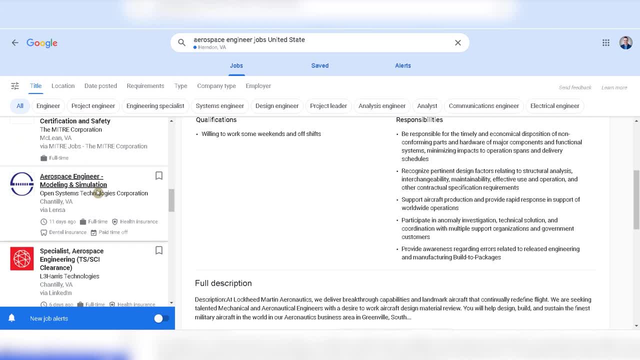 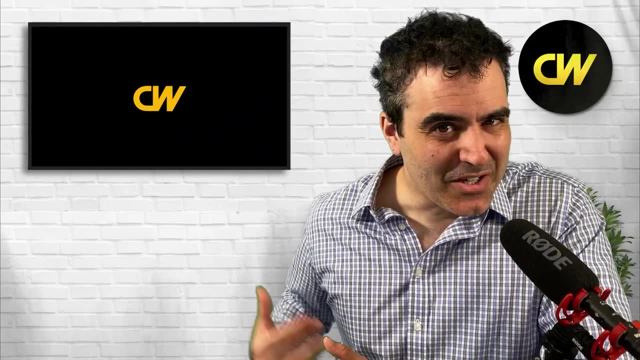 a clearance. Just scrolling through the job postings you see that many of these job opportunities require a clearance And this is a huge con for becoming an aerospace engineer. And this is kind of unique among many of the engineering fields. I mean, there are a lot of engineers that do end 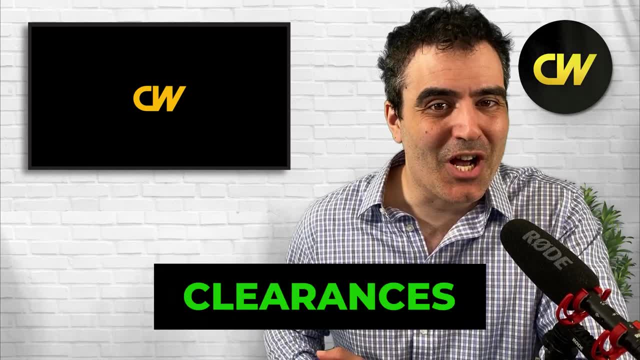 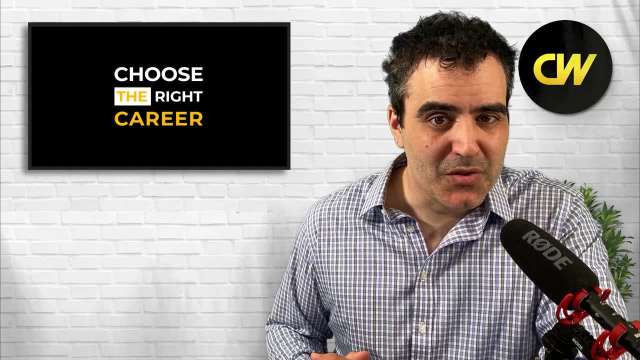 up getting clearances, But for some reason a large portion of the jobs for aerospace engineering, at least in the United States, require some kind of clearance, preventing people from entering those occupations. Next up, we're going to talk about wages, And aerospace engineers actually make a really good. 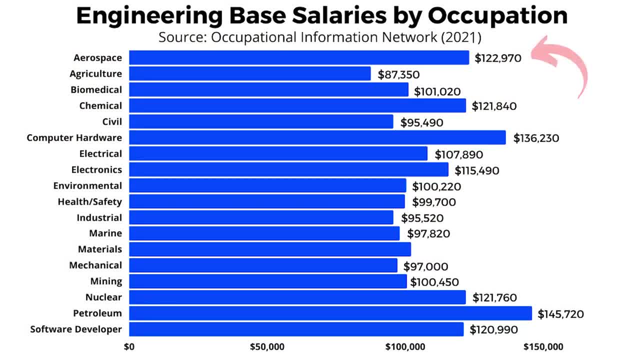 wage In 2021, the average base salary was $122,970 for aerospace engineers. This makes it the third highest paying engineering field. even including software developers, It only falls behind petroleum engineering and computer hardware engineering in terms of base salary. Now, unfortunately for aerospace engineering, the wage growth has slowed down a little bit, and there's other engineering fields that have a greater wage growth, So some of these other engineering fields might catch up to aerospace engineering. In 2016,. the average base salary 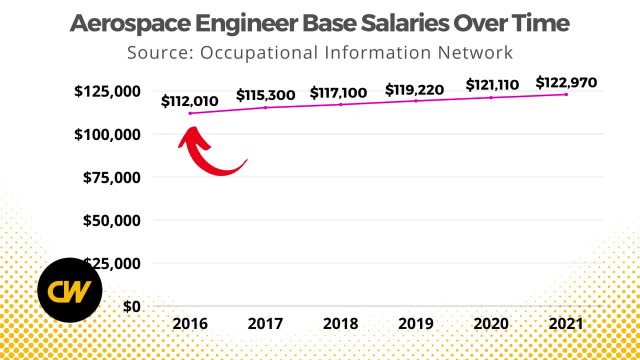 for an aerospace engineer was $112,010.. This grew to $122,970 in 2021. This gives us a 2020 to 2021 wage growth of around $1,800, or a 1.5% raise between 2020 and 2021. And just like every other occupational heritage job, there's a certain hotspot in the first יטing the job anyways. So it's really interesting to see what this Labrador Lazarus program does where we can make things cheaper, even though it might be a little bit more expensive overall. But 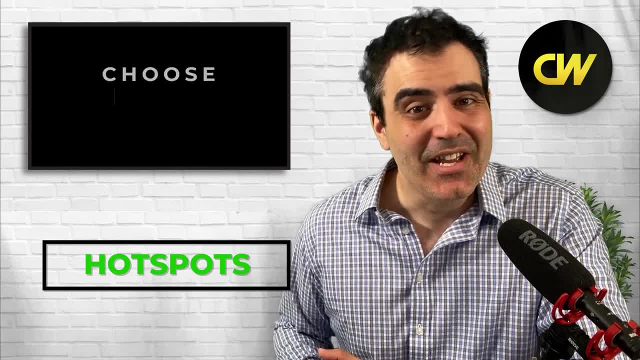 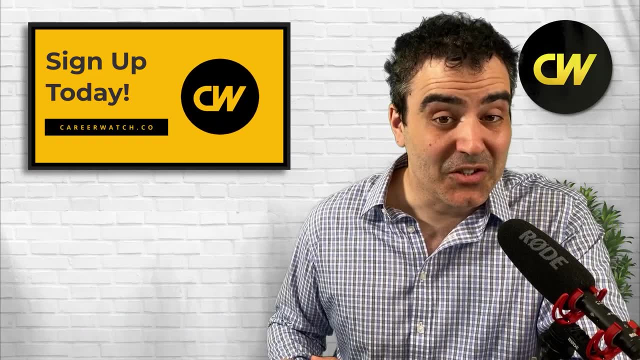 for aerospace engineers, where the wages are way higher than the average across the country. The highest paying place in the country for aerospace engineers is no surprise: It's Silicon Valley, San Jose and San Francisco, California. The average base salary for an aerospace engineer. 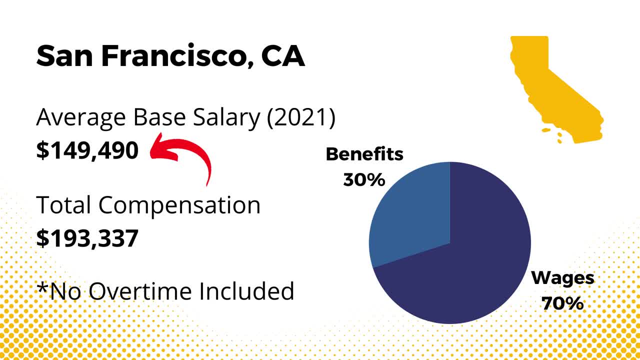 in San Francisco was around $150,000 per year. When you factor in benefits- basically I usually calculate 30%- That's usually how it works- Brings total compensation to almost $200,000 a year for an aerospace engineer in San Francisco. Another hotspot would be the Washington DC area, The 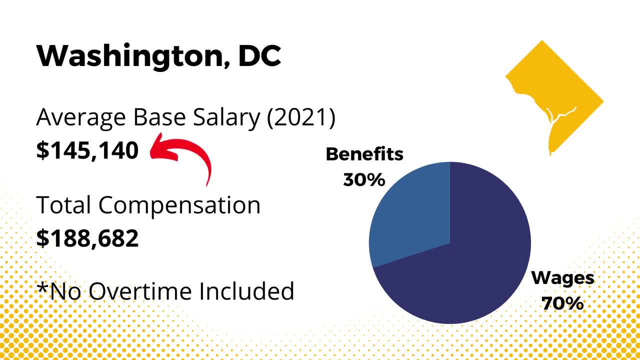 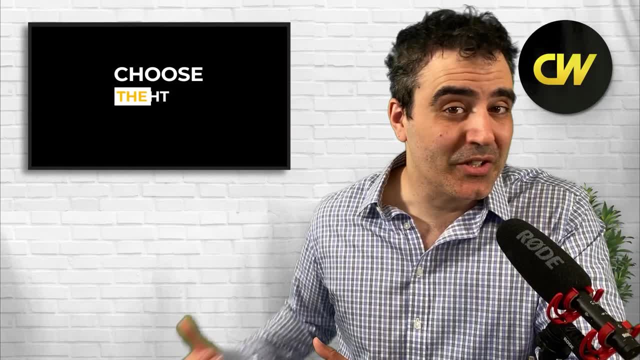 average base salary for an aerospace engineer in DC is around $145,000.. With benefits, this brings total compensation to around $189,000 per year. Now one of the issues of working in DC is you most likely will have to get some kind of clearance for the local jobs in that metro area So that 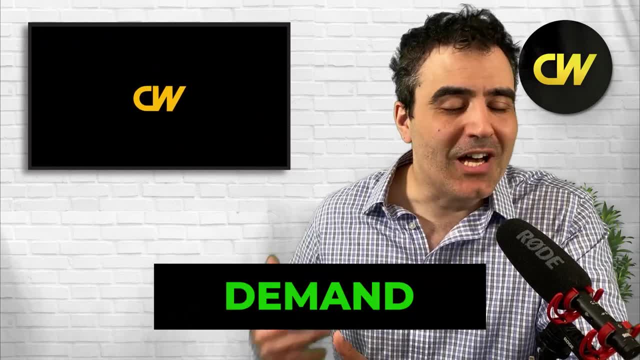 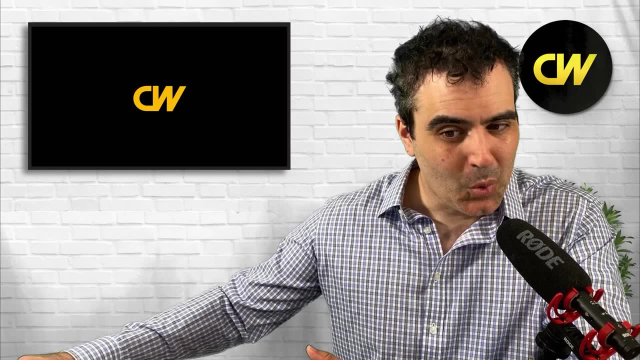 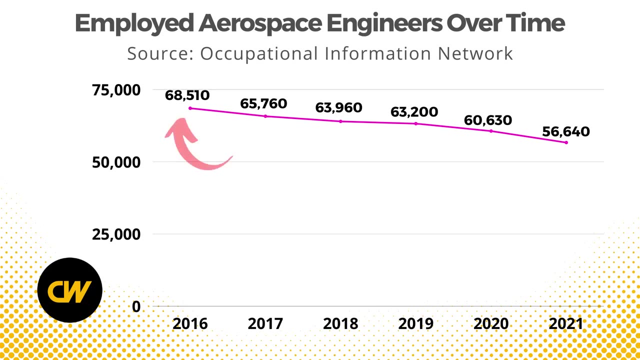 covers wages of aerospace engineers. What is demand like? Is there a lot of demand for aerospace engineers? Unfortunately for aerospace engineers, there's a lot of demand for aerospace engineers. According to the government numbers, the number of employed aerospace engineers has been falling since 2016.. In 2016,, the government recorded around 69,000 employed aerospace engineers By 2021,. 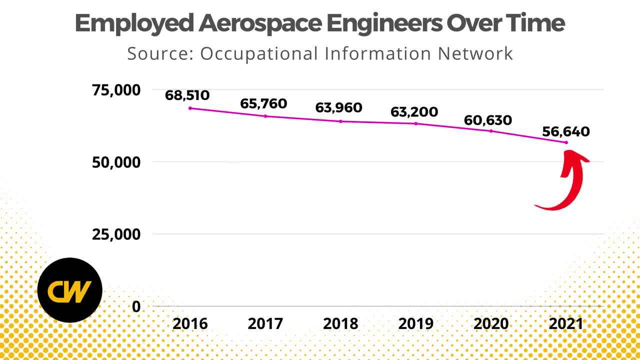 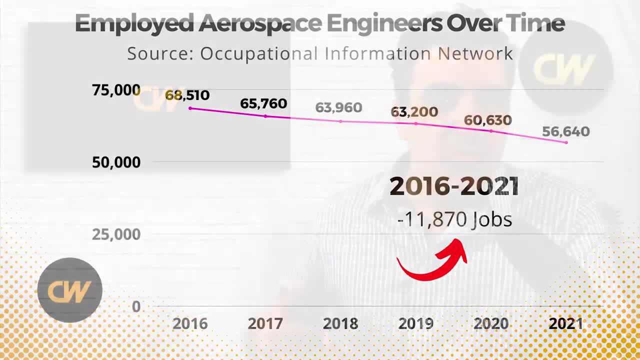 this reached around 57,000.. So between 2016 and 2021, there was a loss of around 12,000 aerospace engineers, according to the Bureau of Labor Statistics. So those are the government numbers regarding the employment of aerospace engineers. They don't look that great. 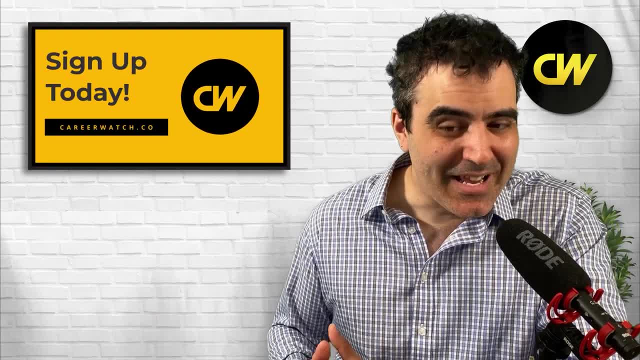 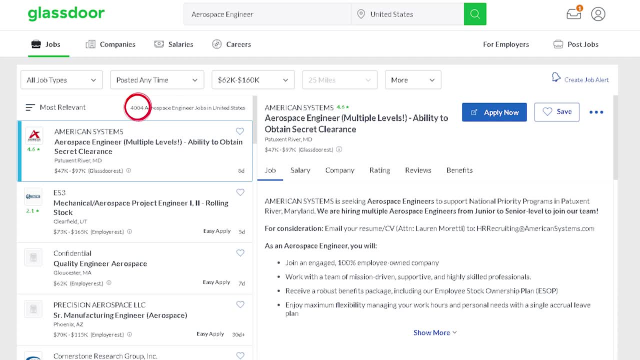 It's terrible when an occupation loses people. That means the jobs get more and more competitive, But according to job postings, they're not really showing the same thing. When I searched for aerospace engineer on Glassdoor, I found around 4,000 job postings. On Indeedcom, 8,500 job. 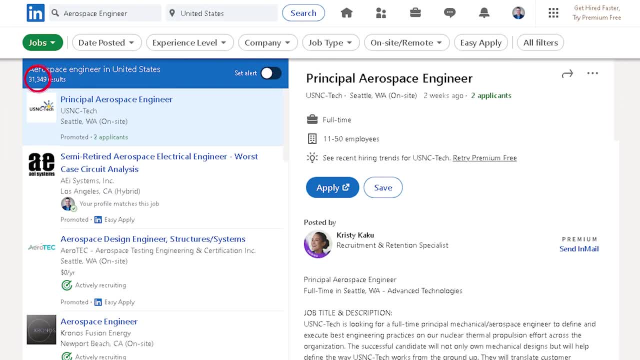 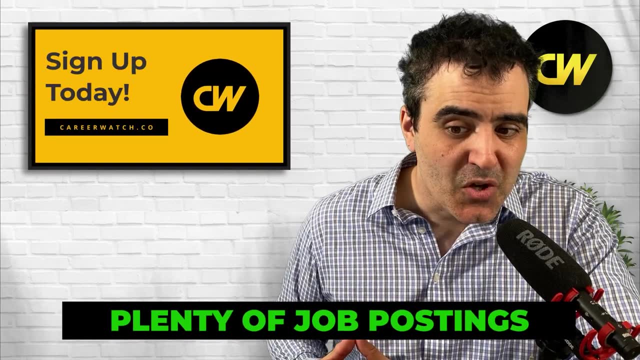 postings And on LinkedIn, 36,236 job postings. So based off job postings, it doesn't look that bad. There's plenty of job postings related to aerospace engineers on Glassdoor, LinkedIn and Indeed. I think the issue here is. 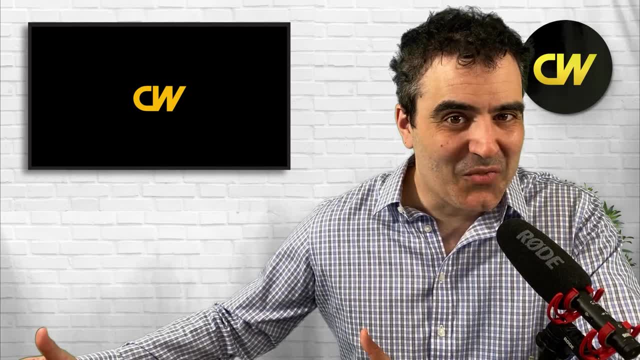 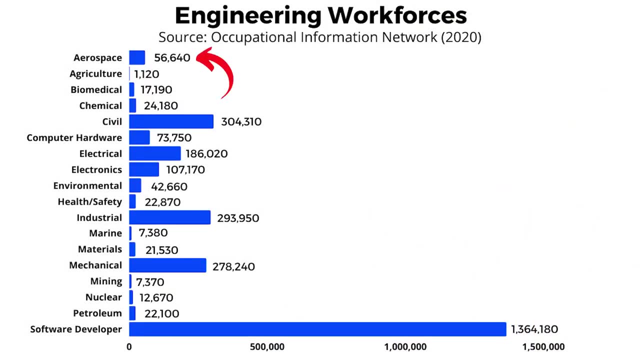 a lot of aerospace engineering jobs might be like reclassified as maybe mathematician or software developer, And you can really see this in the job statistics. There's around 57,000 employed aerospace engineers. There's about 1.4 million software developers in the United States. 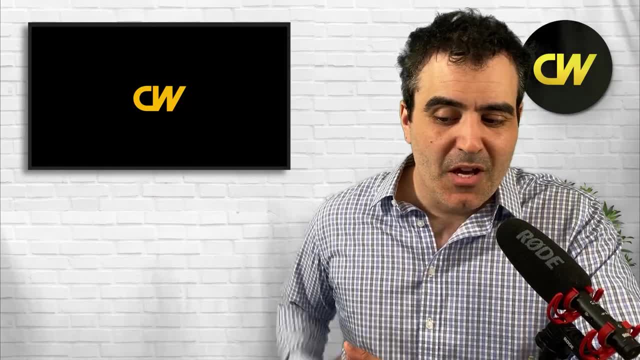 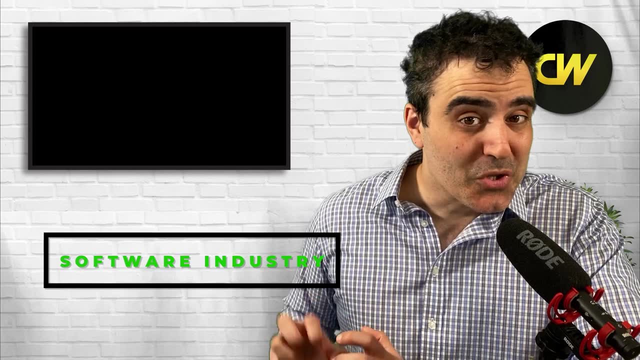 So it's possible that some of those aerospace engineering job opportunities might be kind of reclassified as software developers. But either way, this is kind of the trend. More and more engineers are getting poached by the software industry. Software developers make a great wage and they love to hire people with engineering backgrounds. 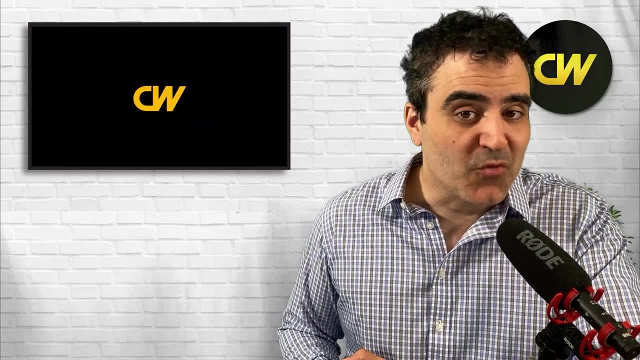 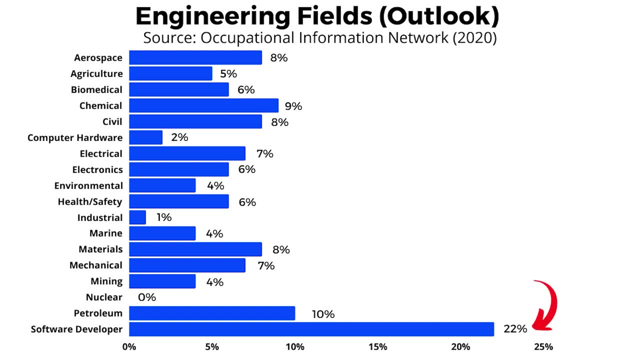 The software industry is just growing by leaps and bounds and the government doesn't forecast it slowing down at all. In fact, when you look at the outlook of different occupations, the government is expecting a 22% increase in software developers over the next 10 years. And